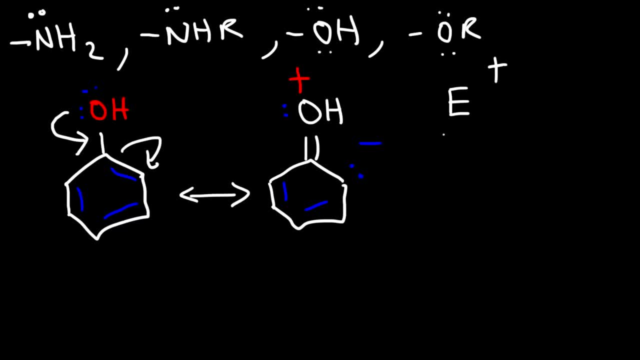 Now, because that carbon atom is nucleophilic, it can react with an electrophile at that position. So thus the OH group is an ortho-director, and if we draw the resonance structure we can put a negative charge on the para-carbon. 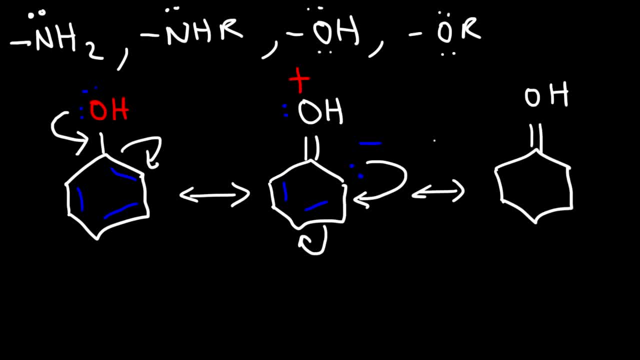 So, whenever you have a strongly activating group, such as an OH group or an OR group, you could see why these groups are ortho-para-directors: because they could put the negative charge on the ortho-carbon, the para-carbon or this one too, which is also ortho with respect to the OH group. 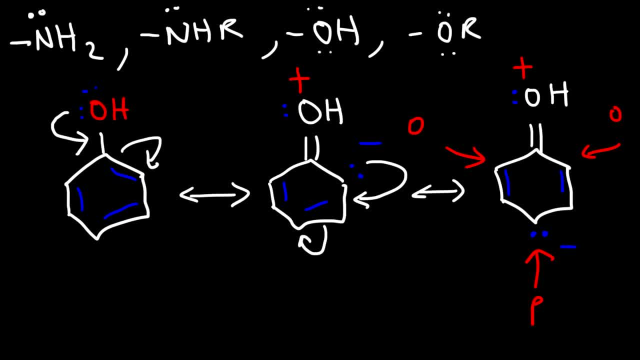 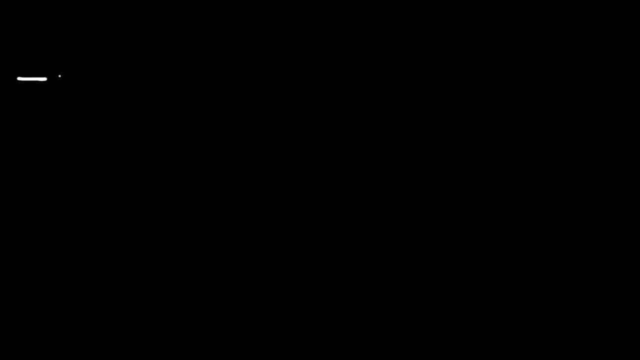 So strongly activating groups are ortho-para-directors and they can donate electrons by means of the resonance effect. Now let's move on to the moderately activating groups. So these include the amide and the ester functional groups. So this is the amide and the ester functional group, where the benzene ring is attached to the oxygen part of the ester. 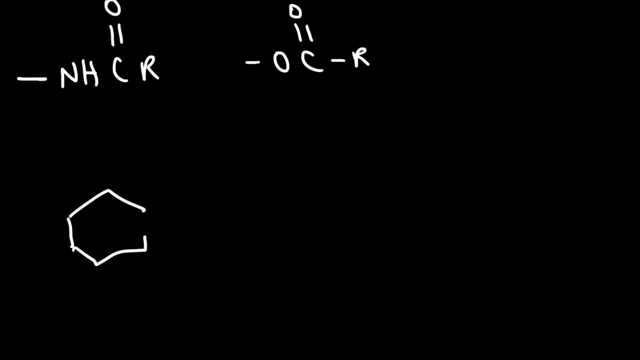 So let's use the ester as an example. So for the moderately activating groups, they can still donate electron density by means of the resonance effect. So therefore they're going to be ortho-para-directors. As you can see, we can put the negative charge on the para-carbon. 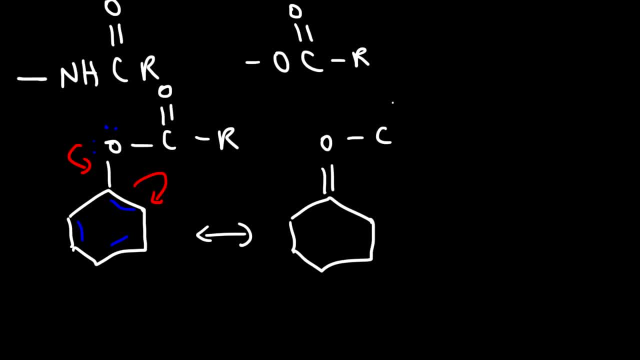 The ortho-carbon, just like we did in the last example. Or we could put the negative charge on the para-carbon if we draw the resonance structure. So moderately activating groups are ortho-para-activators. Now why are they called moderately activating? 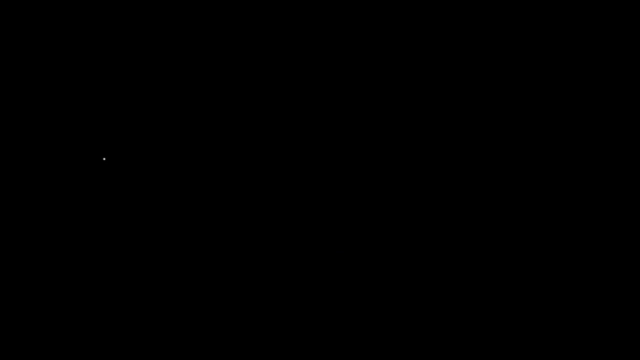 Why are they not strongly activating? So if we start with this structure, notice that the carbonyl group pulls on the lone pairs of the oxygen So as a result, it's less effective in donating electrons to the ring, but it still can do so. 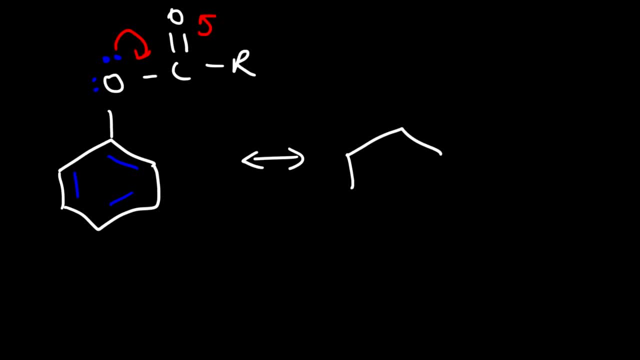 So that's why it's not strongly activated, It's moderately activated. Next on the list we have the weakly activating groups. These include an alkyl group or another aromatic ring or, let's say, a venal group, And so these are weakly activated. 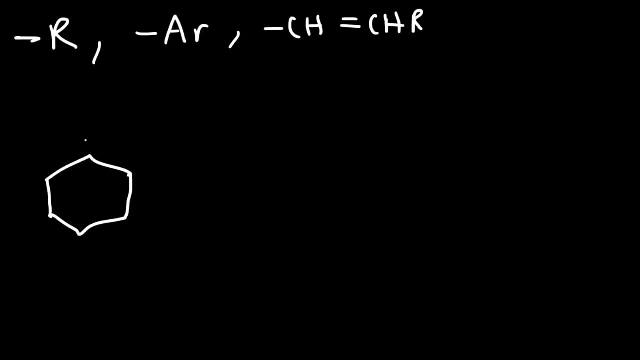 Let's focus on the weakly activating groups. Let's focus on an alkyl group such as a methyl group. So here we have toluene, And the methyl group cannot donate electrons by means of the resonance effect. The carbon doesn't have a lone pair. 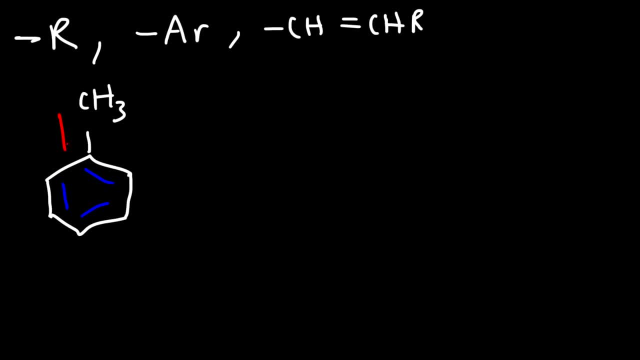 So all it can do is donate electron density inductively, That is, through the sigma bond. So is the methyl group an ortho group, Like I mean, is it an ortho-para-director, Or is it Or is it a meta-director? 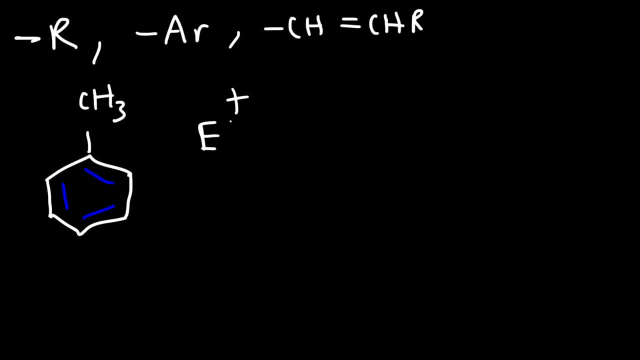 Well, let's find out. So let's react this with an electrophile. If we put the electrophile, let's say, on the ortho-carbon, let's see what's going to happen. So here is the electrophile. 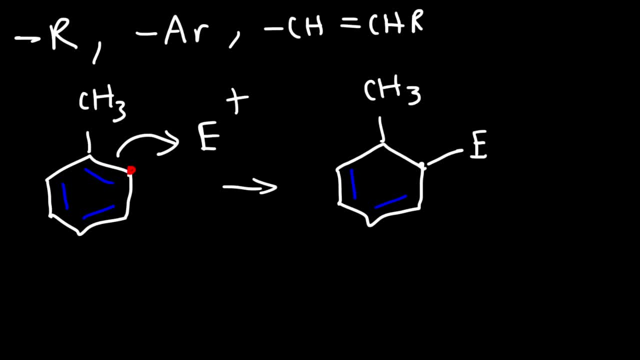 And we lost the double bond. so we have two double bonds And since we put the electrophile on this carbon, the positive charge has to be on this carbon. So notice that this is the best place where we can put the positive charge on this ring. 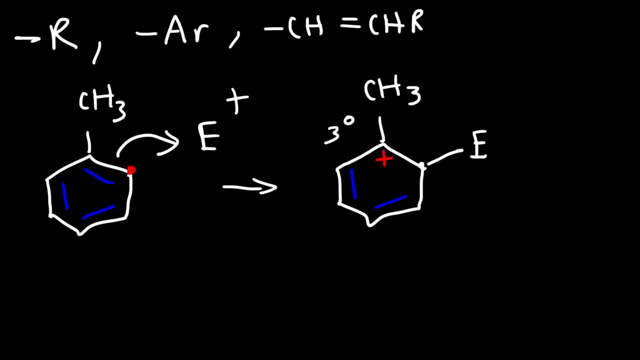 because that's a tertiary carbocation as opposed to a secondary one. Now let's say, if we put the electrophile in the meta position, Let's see what's going to happen. So here is our methyl group. So this double bond here has been unaffected. 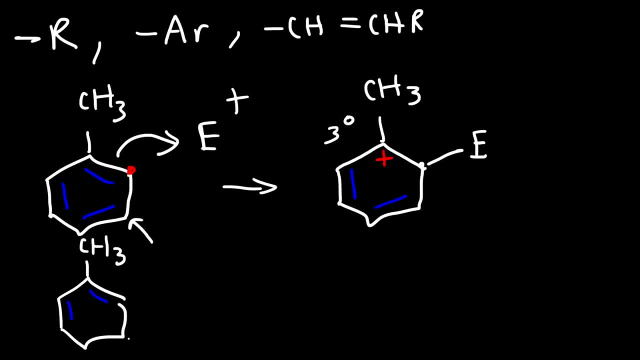 Now we're going to lose this double bond. So if we put the electrophile, If we put the electrophile on the right side of that double bond, the positive charge has to be on the left side. Now let's draw the resonance structure for this carbocation. 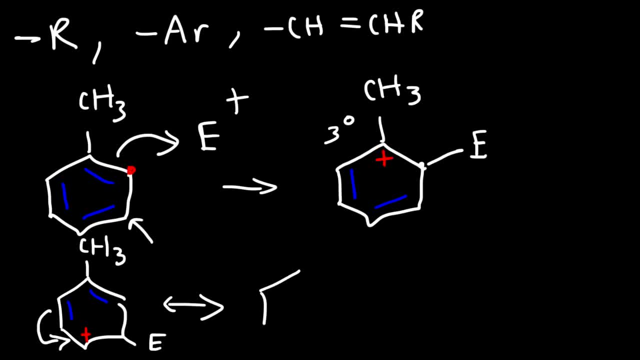 So we can move this double bond here, giving us this group. And so now the double bond is in this region And notice that we still have a secondary carbocation. Now let's draw. Let's draw another resonance structure. The plus charge is going to jump by two carbons each time. 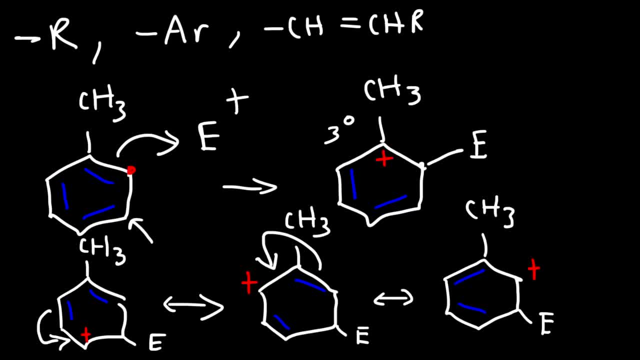 So notice that we miss the tertiary carbon. So if we put the electrophile on the meta position- this is the ortho position, this is meta, this is para- we won't get a tertiary carbocation. Now what if we put the electrophile on the para position? 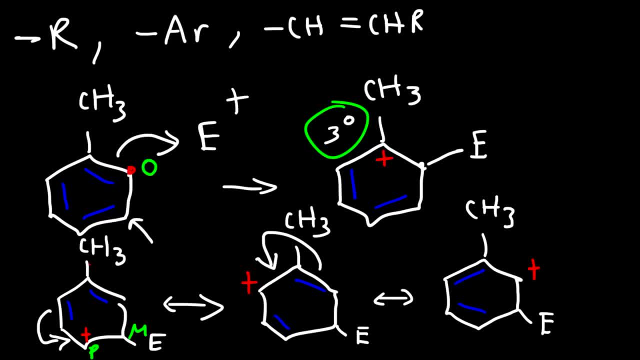 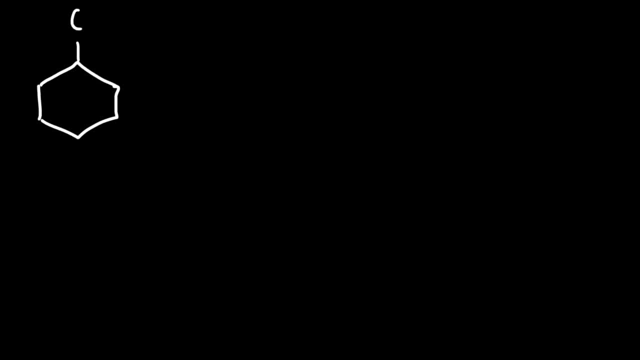 Will we get a stable tertiary carbocation? So let's find out. So let's start with the original toluene molecule And so we're going to react the electrophile Using this double bond and we're going to put it in the para position. 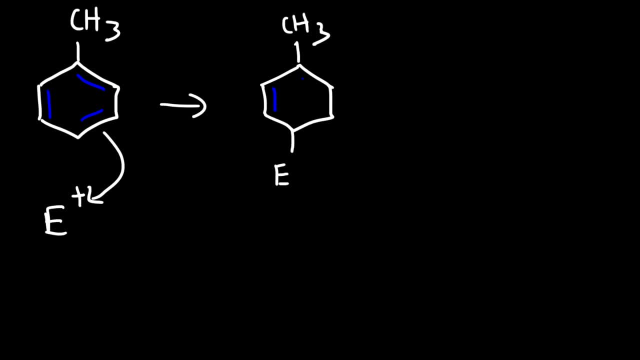 So here it is. The double bond on the left and at the top have been unaffected. So if we put the electrophile here, the positive charge has to be on the other carbon. And now let's move this double bond towards that positive charge. 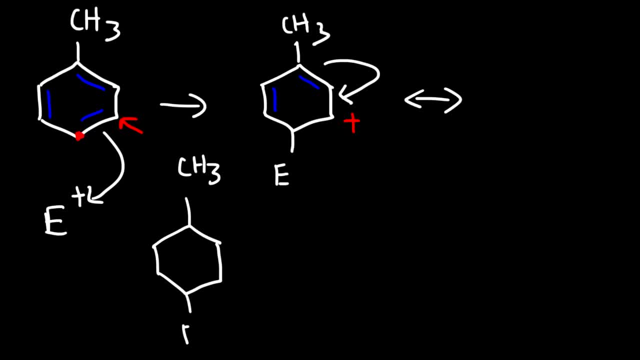 And so the positive charge and the double bond. they're going to trade places, And so notice that we now have the positive charge on the tertiary carbon. And so if we place the electrophile on the ortho position or on the para position, 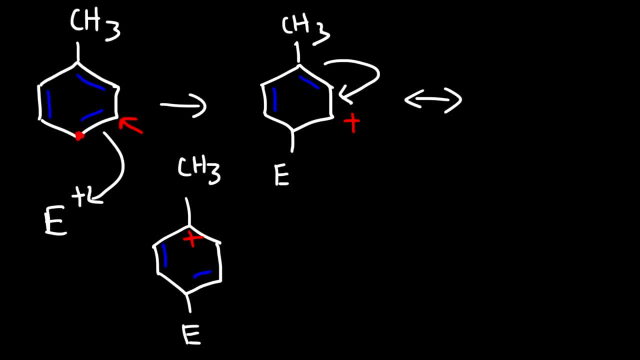 it led to a stable tertiary carbon, Whereas if we put it on the meta position, we got a secondary carbon with a positive charge, And so we can see that there's no positive charge. And so we can see why, if we add a methyl group to a ring or an alkyl group, why the alkyl group is an ortho-para-director. 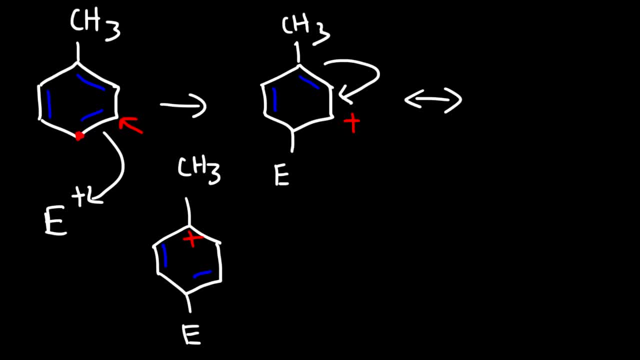 Because putting the electrophile in that position will lead to a more stable carbocation intermediate. Well, technically you can call this like a sigma complex or an arenium ion, But it's better to have a positive charge on a tertiary carbon rather than a secondary carbon. 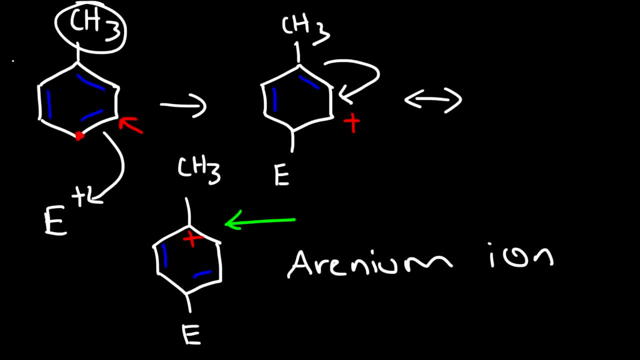 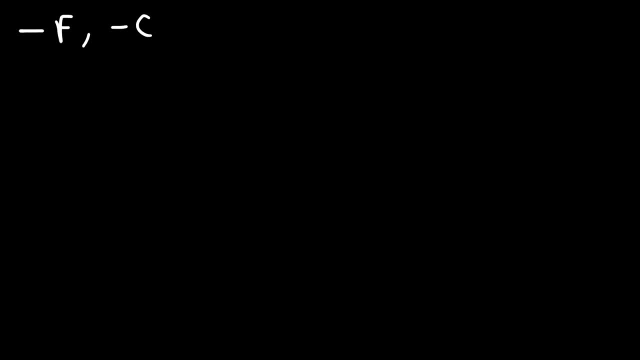 And so that's why this methyl group is an ortho-para-director. Now let's move on to the weakly deactivating groups. So these include the halogens like fluorine, chlorine, bromine and iodine. 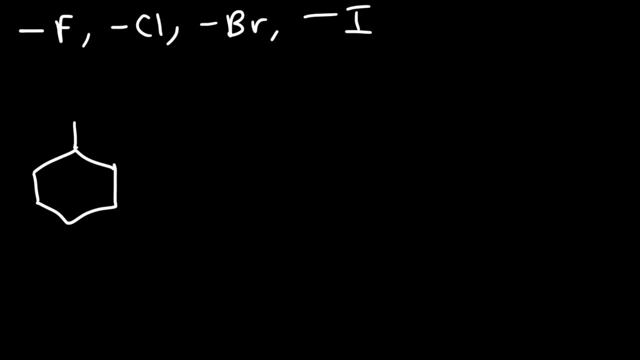 Let's use bromine as our example. Now, why are these groups called weakly deactivating? Why do they deactivate the ring? Why do they make it less nucleophilic? The halogens can do two things. First, you need to realize that these atoms are electronegative atoms. 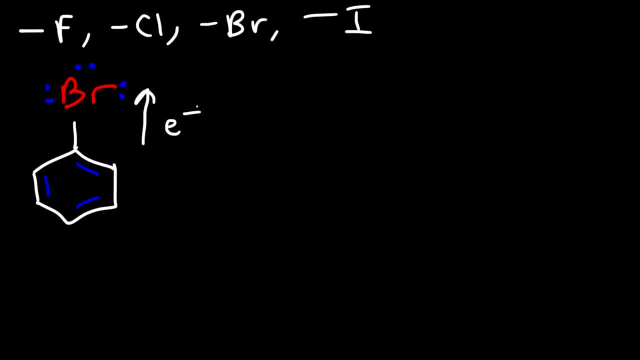 And so they can pull electrons away from the ring by means of the inductive effect, that is, through the sigma bond, But at the same time they can donate electrons to the ring by means of the resonance effect, because they do have lone pairs. 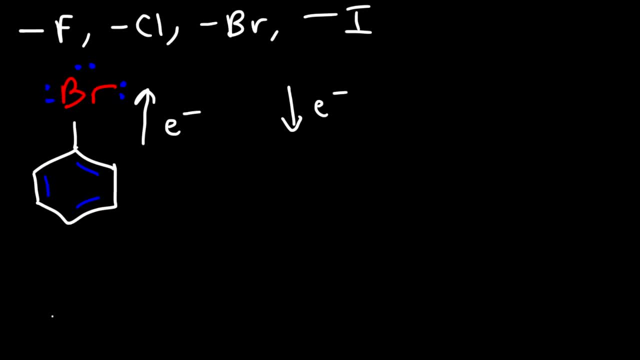 And so their electron withdrawal effect- let's call it EWG- exceeds their electron donating effect. So they can behave as an electron withdrawing group and as an electron donating group. So because their withdrawal effect is greater than their donating effect, 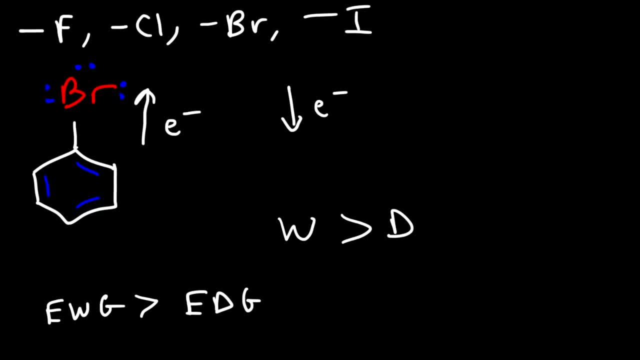 these are weakly deactivating groups. Now, in the case of a strongly activating group, let's say, like phenol, which we used earlier in this video, the oxygen atom is an electronegative atom And so it can withdraw electrons inductively, but it does have lone pairs, so it can donate electrons inductively. 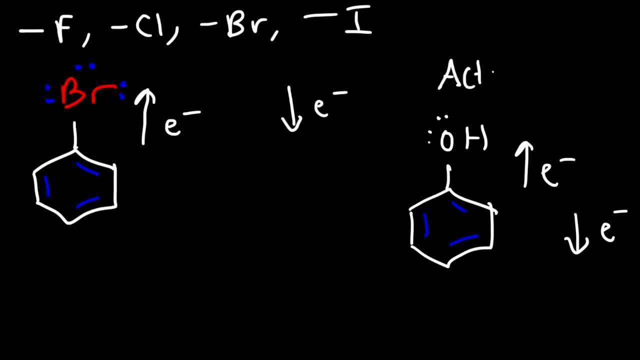 However, this is an activating group, So that tells us that its donating effect exceeds its withdrawn effect. But since this is a deactivating group, its withdrawn effect exceeds its donating effect, And so it's important to understand that concept. And now let's get back to bromobenzene. 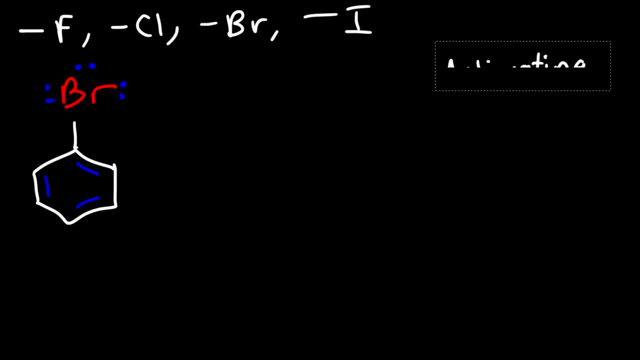 The halogens. even though they're weakly deactivating, they're still ortho-para-directors, And the reason for this is because they have lone pairs, And so they can donate electron density to the benzene ring by means of the resonance effect. 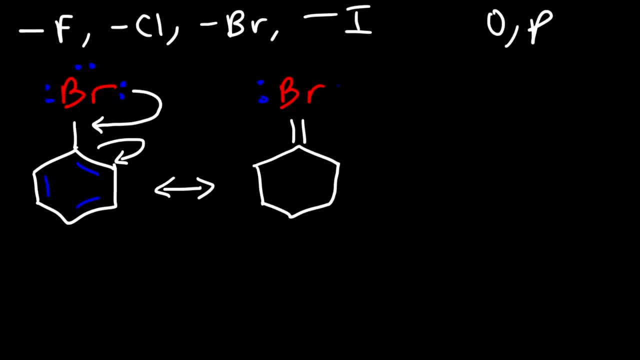 In this resonance form, bromine has two lone pairs and a positive charge, But now notice that it puts a negative charge on the ortho-carbon, making the ortho-carbon more nucleophilic, And they could also put a negative charge on the para-carbon. 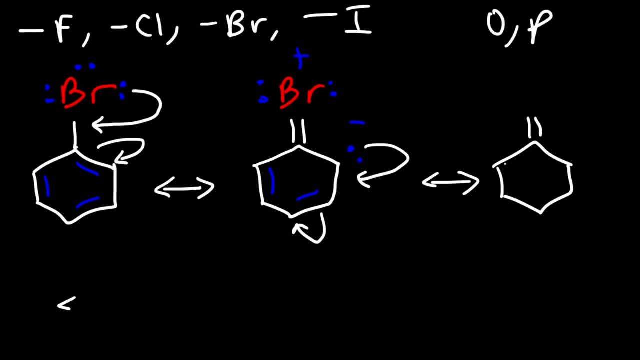 making that carbon nucleophilic. And so we could see why the halogens are ortho-para-directors, Because by means of the resonance effect they can put a negative charge on the ortho-carbon and on the para-carbon. 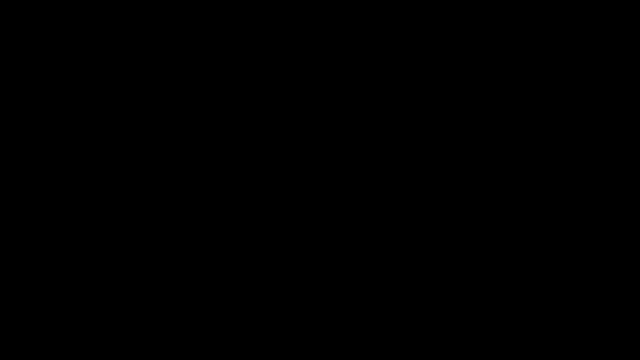 Next up we have the moderately deactivating groups. So these include the aldehyde functional group, the ketone, the ester, But this time the benzene ring is attached to the carbonyl group of the ester and not the oxygen. 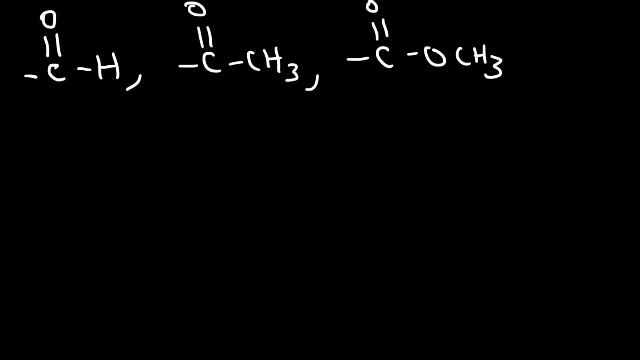 Because, if it was, it would be moderately activated as opposed to moderately deactivated. And the other one is when it's attached to a carboxylic acid. So if you have a benzene ring attached to a carbonyl group, as you can see, in most of these cases it's a moderately deactivating group. 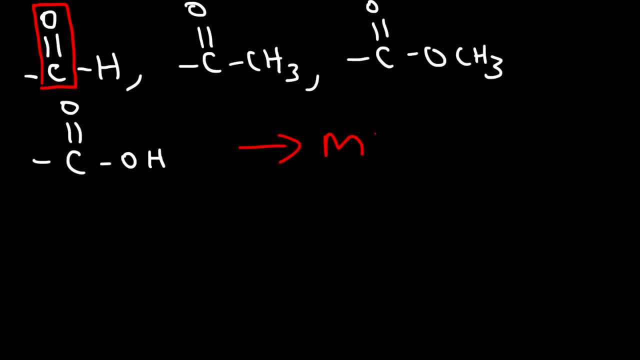 Moderately deactivating groups are meta-directors. They can withdraw electrons by means of the resonance effect. Next up, we have the strongly deactivating groups like the nitro group, cyanide, a nitrogen with three R groups and a positive charge. 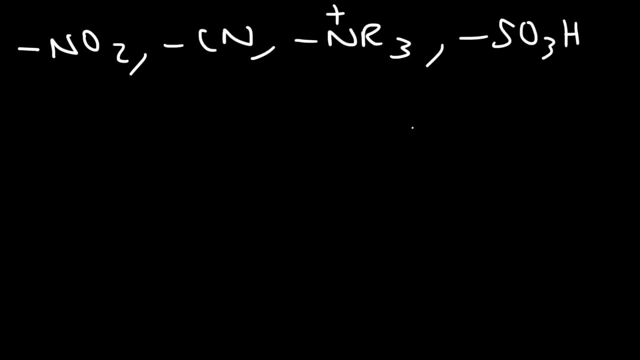 or the sulfonic acid group. So these can also withdraw electrons by means of the resonance effect, And so they're meta-directors. Now let's use NO2 as an example. So it has two oxygen atoms attached to it, And the nitrogen atom has a positive formal charge. 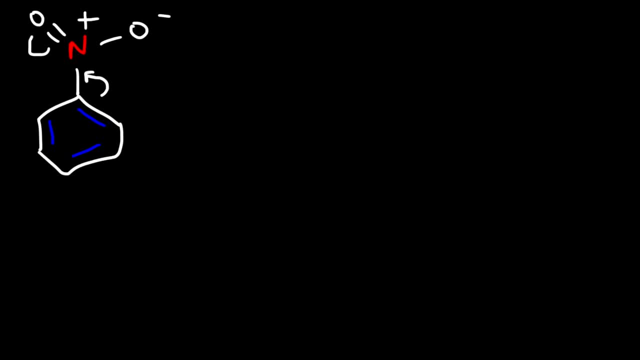 So the nitro group can pull electrons toward itself, put in a positive charge on the ring And as a result, it makes the ring less nucleophilic, more electrophilic, And so therefore it doesn't want to react with an electrophile. 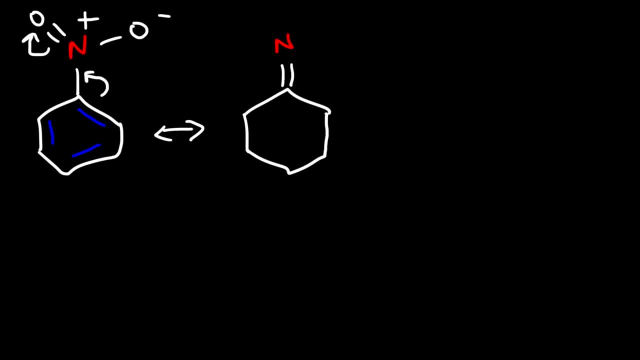 Thus, the ring is deactivated towards electrophilic aromatic substitution reactions. However, if you're dealing with nucleophilic aromatic substitution reactions, then this is a good thing. It'll make the ring more reactive towards nucleophilic aromatic substitution reactions. 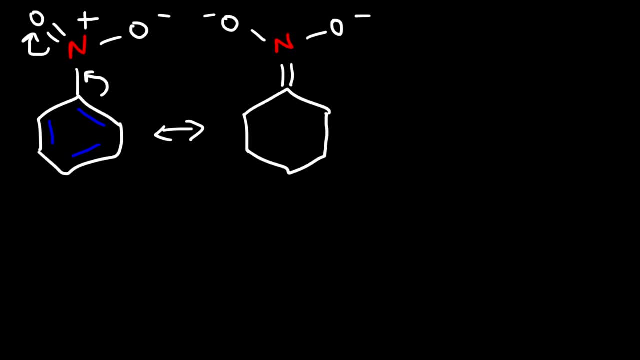 but it makes it less reactive to electrophilic aromatic substitution reactions, Which is usually what we're dealing with. So notice that we have a positive charge on the ortho carbon And so that carbon does not want to react with an electrophile. 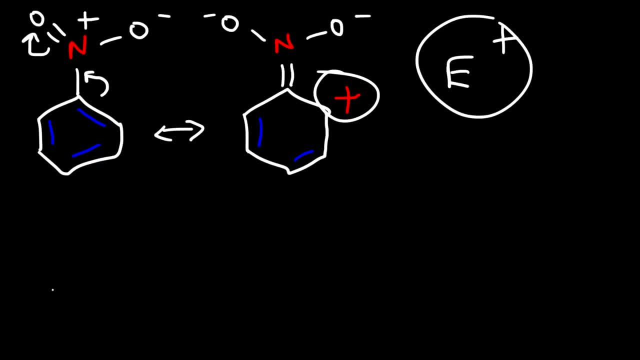 because they have the same charge And so they repel each other. Now let's take this double bond and move it here, Generating a new resonance structure. So notice that the positive charge is on the para carbon, So both the ortho carbon and the para carbon. 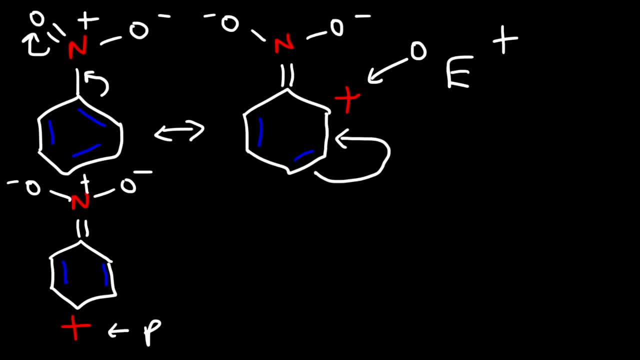 they're electrophilic. The only carbon that's not electrophilic in this example is the meta carbon. As you can see, we can't put a positive charge on the meta carbon, So therefore that's the most nucleophilic carbon in this ring. 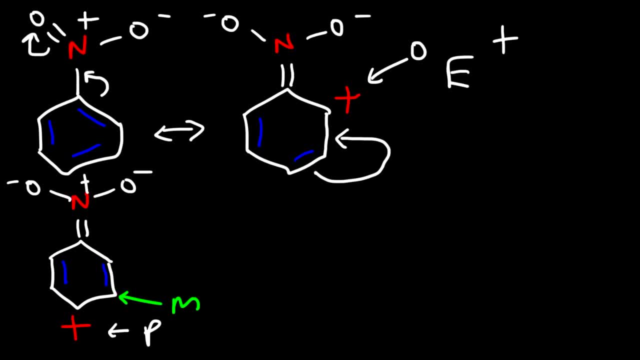 A neutral atom is more nucleophilic than an atom with a positive charge, So, as a result, this is the only atom in a ring that is most likely to react with an electrophile. Therefore, strongly deactivating groups are meta directors.